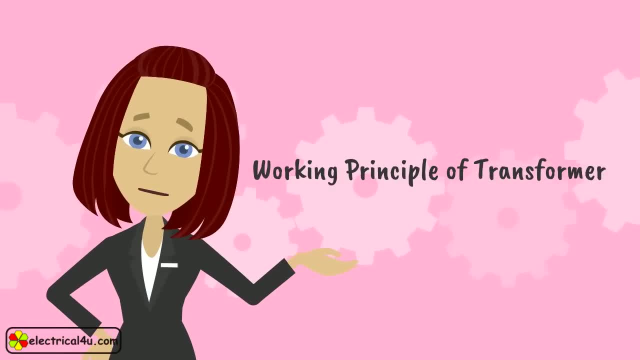 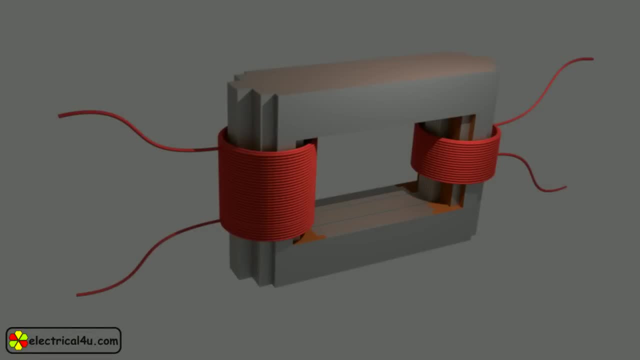 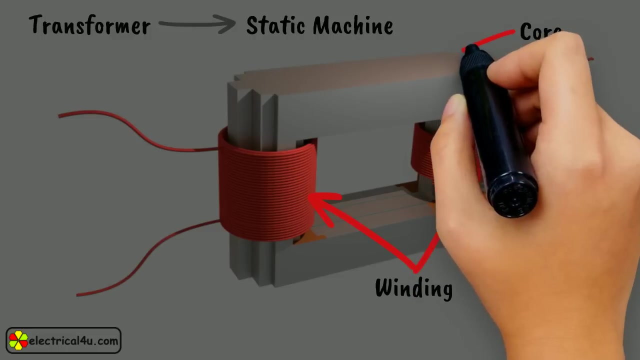 The working principle of transformer. Actually, transformer is a machine, but it does not have any moving part. That is why a transformer is referred to as a static machine. A transformer has three main parts: Two windings and a metallic core on which the windings are wound. 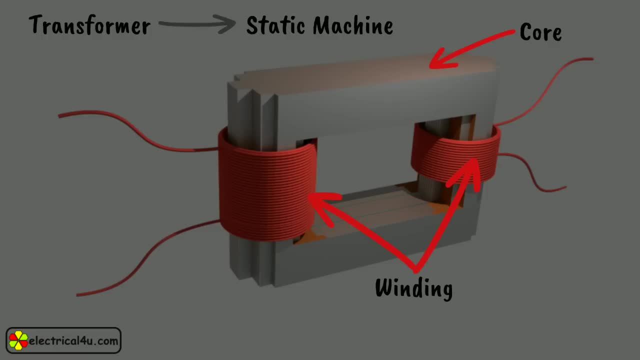 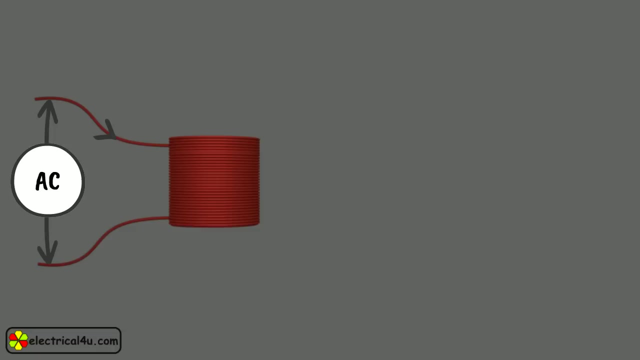 Windings are in the form of coil, made of a good conductor of current. The windings of a transformer play a main role in the machine. The winding coils behave as an inductor. When an alternating current is allowed to flow through any of the windings, there will be an 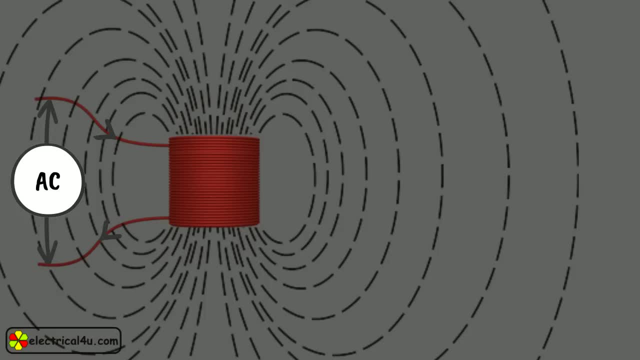 alternating flux produced surrounding the coil. When an alternating current is allowed to flow through any of the windings, there will be an alternating flux produced surrounding the coil. The magnitude of this flux is proportional to the magnitude of the current flowing through the winding. The direction of the flux is according to the direction of current. The direction of. 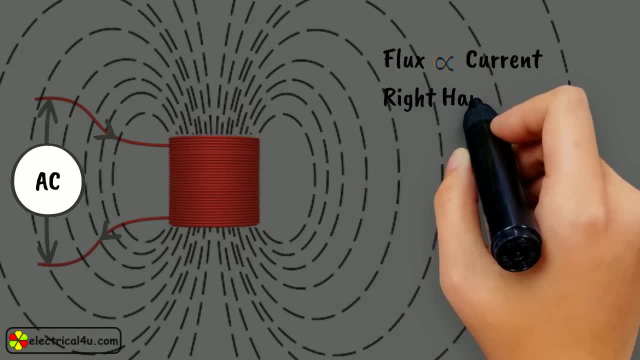 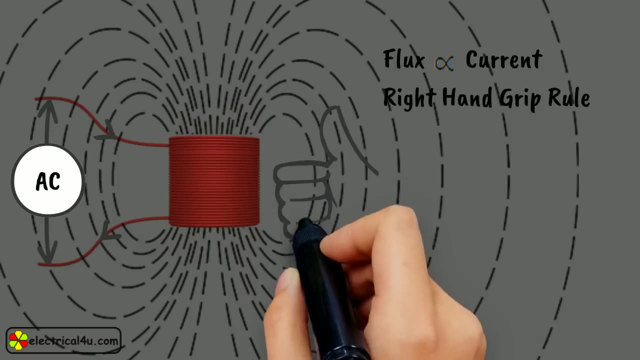 the current in the winding can be found out by applying right hand grip rule. This rule states that when we grip our right hand with stretching the thumb along the axis of coil or winding and other four-fold direction, the direction of the flux will be determined. The direction of the flux. 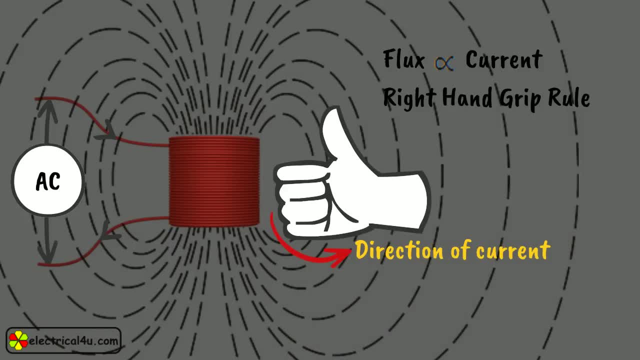 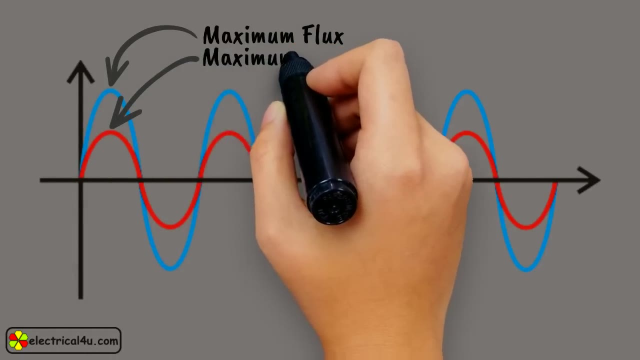 will be indicated by the index finger pointing to the direction of the current in the coil. Then the thumb indicates the direction of produced flux inside the coil along the axis. This flux becomes maximum in magnitude when current reaches its maxima for one half cycle of alternating. 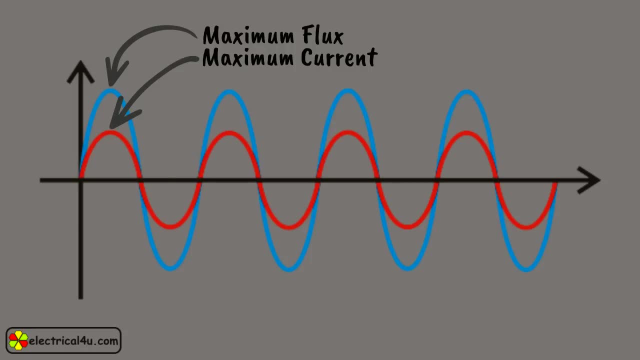 current wave. The flux becomes zero when current in the coil crosses zero axis. Again for next half cycle, the flux is given as zero when current in the coil crosses the zero axis. This is true for every unit of the coil in the coil. 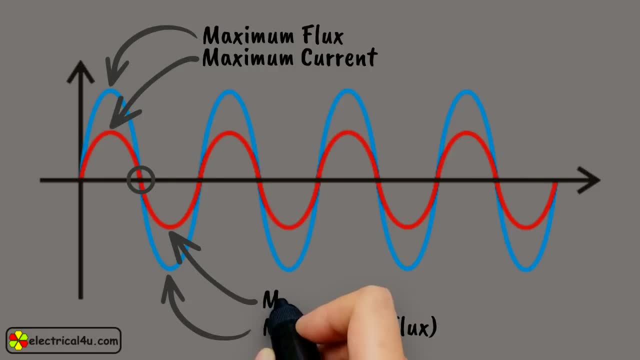 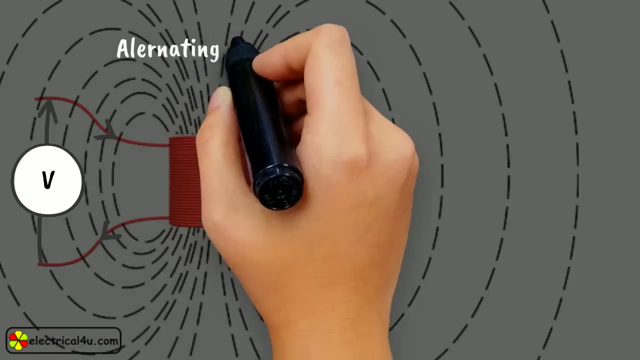 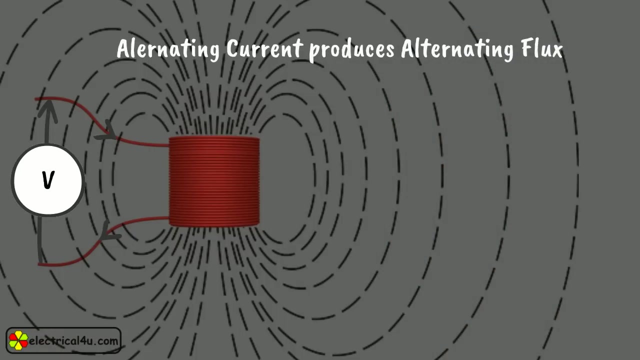 the flux becomes maximum, but in opposite direction, when current reaches to its reverse maxima. In this way, alternating current produces continually varying flux surrounding the winding. The flux lines link the winding itself and the flux is varying, so there will be self-induced EMF across the winding. 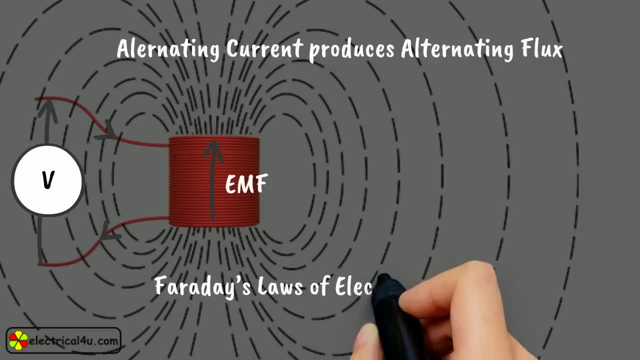 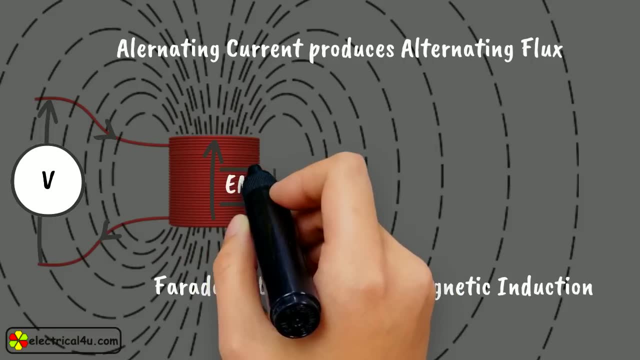 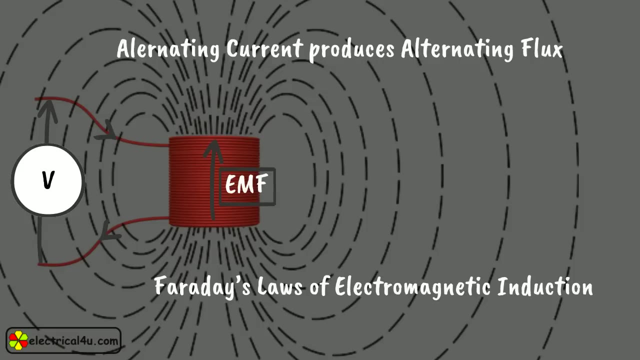 This phenomenon is due to Faraday's laws of electromagnetic induction. This induced EMF or voltage, whatever you say, is same in magnitude and opposite in polarity of supply voltage Supplied. alternating voltage causes alternating current in the winding, which produces continually varying flux inside and outside the winding. 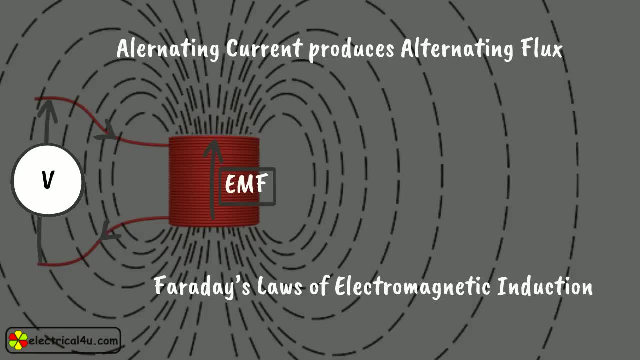 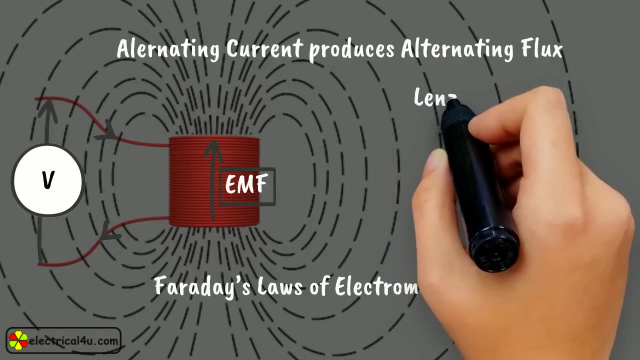 This condition is called the flux line. Continually varying flux produces induced EMF across the winding. So we can say that the supply voltage is caused and induced voltage at the winding is in effect of this cause. Hence, according to Lenz's law, 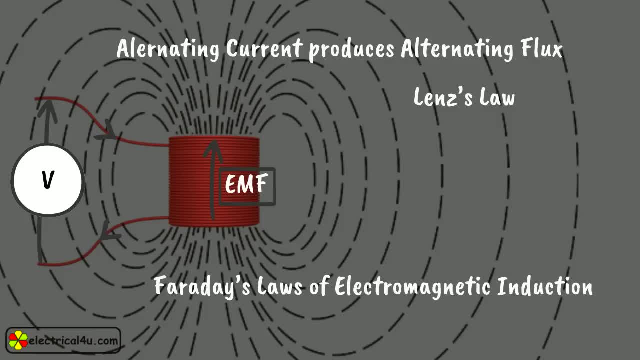 this induced voltage will be in opposite polarity of supply voltage, Since, according to Lenz's law, effect always opposes cause. This self-induced voltage across the winding does not depend upon the number of turns in the winding but depends on the supply voltage. But the voltage induced per turn depends on the number of turns in the winding. 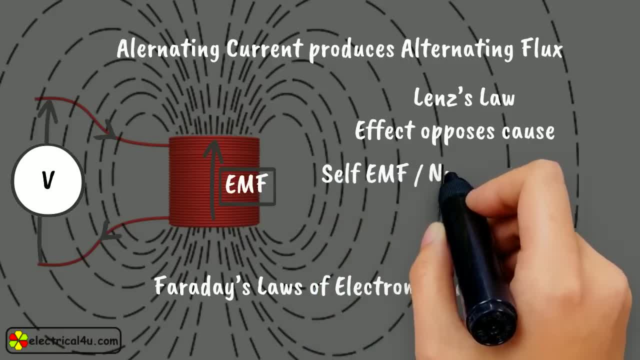 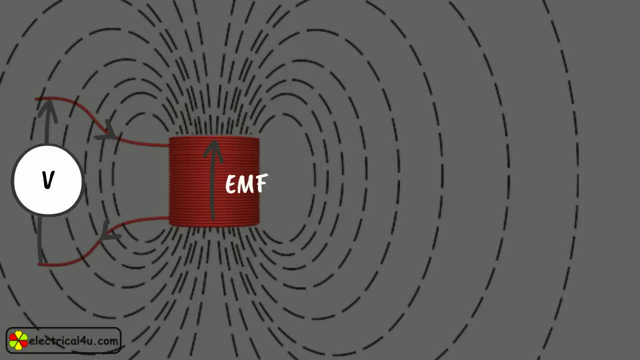 This is nothing but induced EMF divided by the number of turns in the winding. We have said that there is another winding in the most basic transformer, but till now we have not discussed it. Now we are coming to second winding in the transformer, Supposing one separate winding is brought nearer to the first winding. 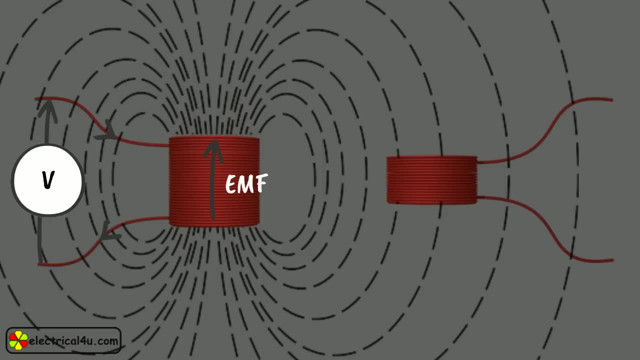 then this second winding gets kinked with a portion of varying flux of first winding. Due to this varying flux linkage, there will also be an induced EMF across it. This induced EMF would be quite small, as because the flux linkage is small, Hence rate of change of flux linkage is also small. 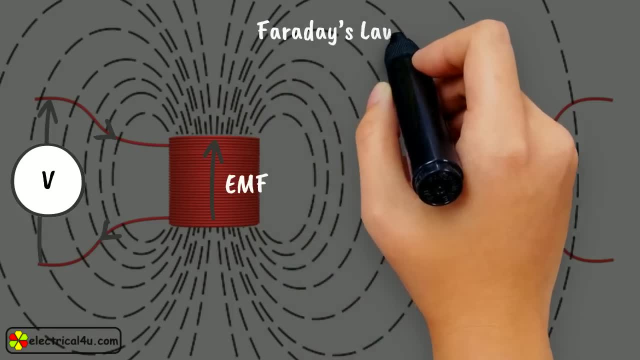 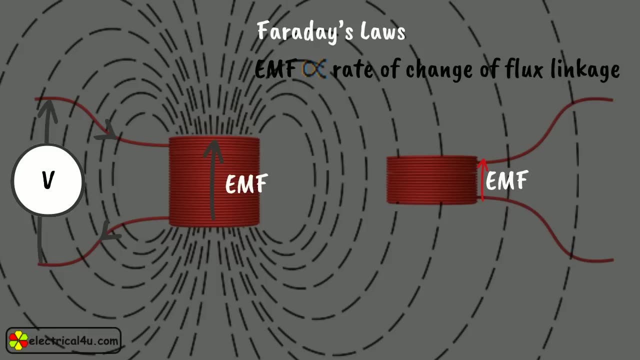 and according to Faraday's laws, induced EMF across a coil is directly proportional to the rate of change of flux linkage. If now we connect a closed circuit across the second winding, we will get a very tiny current through the circuit, provided the second winding is placed much nearer. 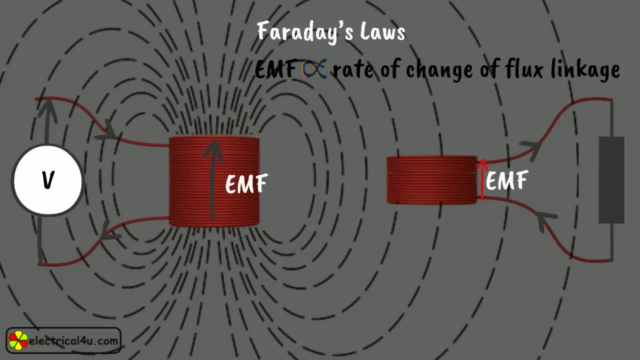 to the first. So we have seen that some portion of the input power is transformed to output through the second winding. This is because some portion of generated flux of first winding is linked with second. Now, if we want to transform maximum electric power from first winding to second winding, 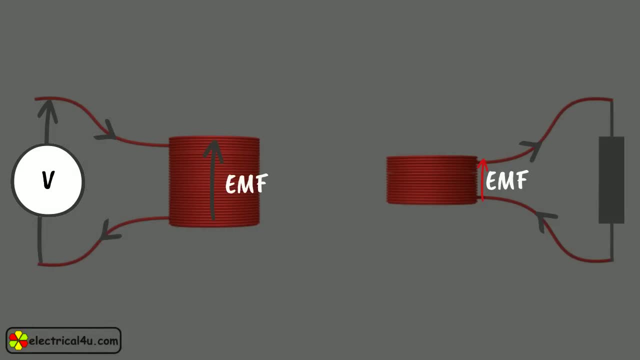 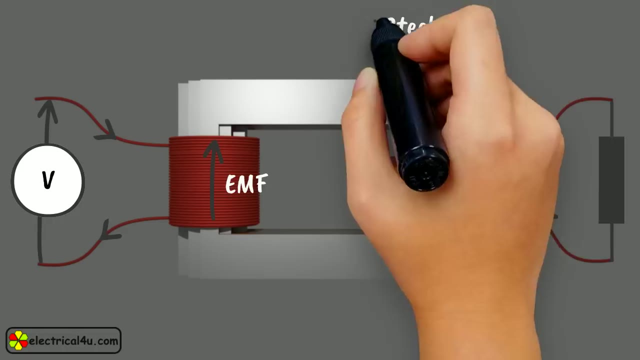 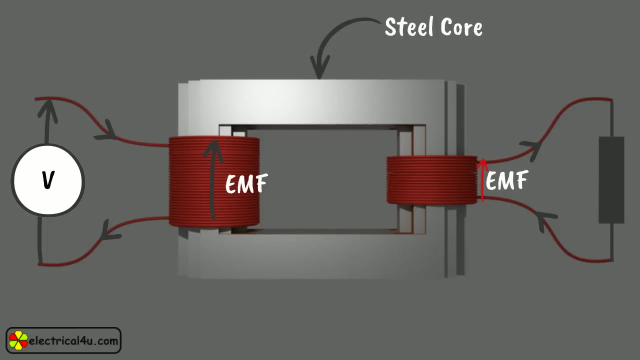 we have to link maximum flux of first winding to second winding. This is done by placing a low reluctant magnetic core in between these windings. Steel is a well known low reluctant magnetic material, So we normally use steel for making low reluctant magnetic core in the transformer. As soon as we place a steel core in between these windings, 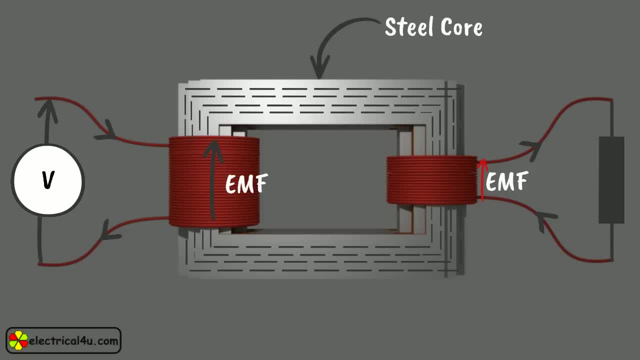 nearly the entire flux which was surrounding the first winding will be concentrated inside the core and leak with the second winding, As nearly the same flux links with second winding. now the rate of change of flux with respect to time is equal in both windings Since, as per Faraday's laws of electromagnetic induction, 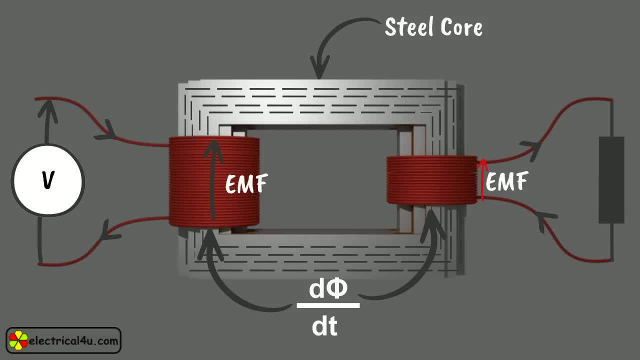 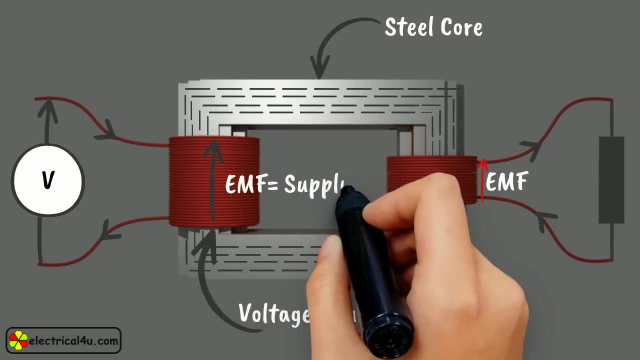 induced EMF across a conductor is directly proportional to the rate of change of flux linkage. The voltage induced per turn in both windings will be the same. We have already explained that voltage induced across the first winding is the same as the supply voltage. Actually, here we consider that there is no voltage drop between supply terminals and the first winding. 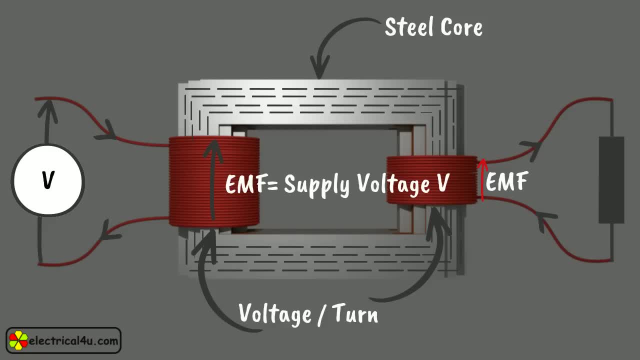 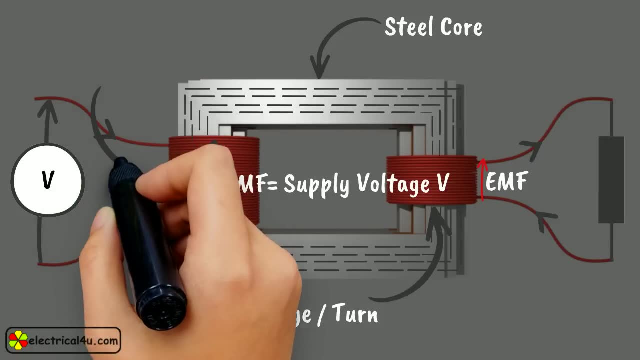 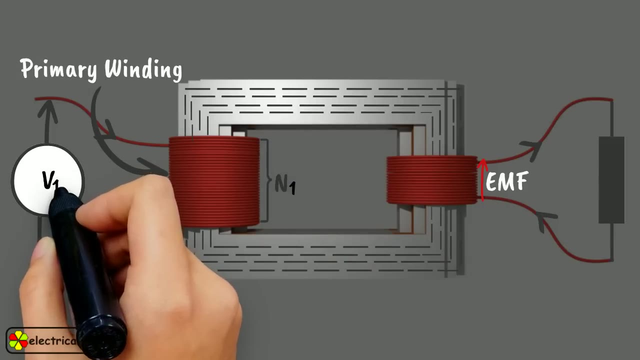 This is an ideal case For theoretical purposes. we will consider that condition. As this first winding is connected with supply, it is referred to as primary winding. Now, if this primary winding has N1 number of turns and supply voltage or induced voltage across primary winding is V1,